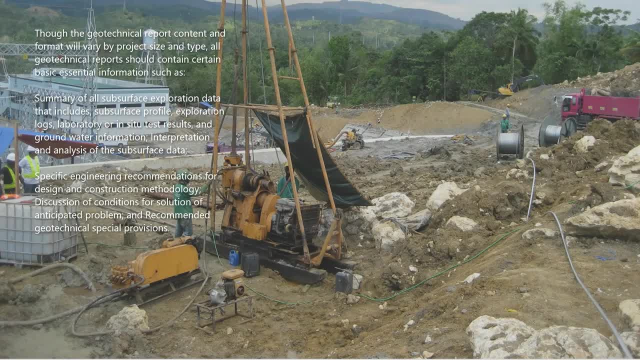 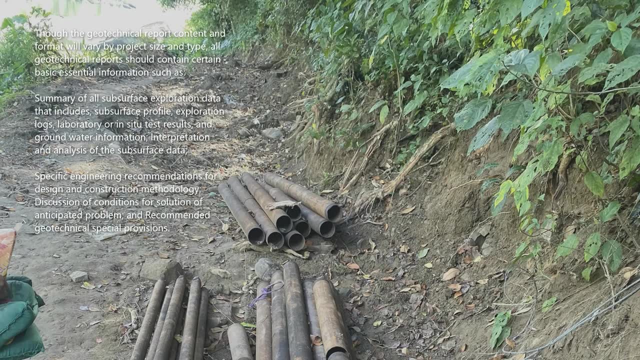 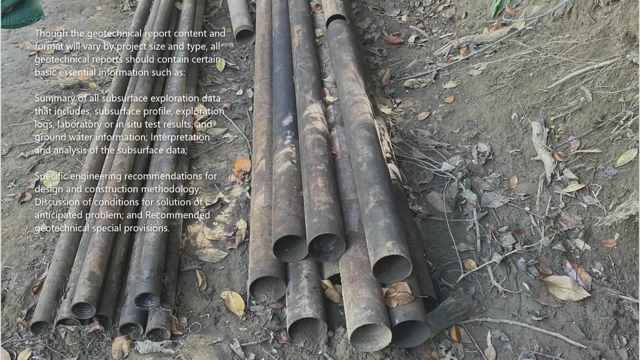 Though the geotechnical report content and format will vary by project size and type, all geotechnical reports should contain certain basic essential information, such as summary of all subsurface exploration data. that includes subsurface profile, exploration logs, laboratory or in-situ test results and ground water information. 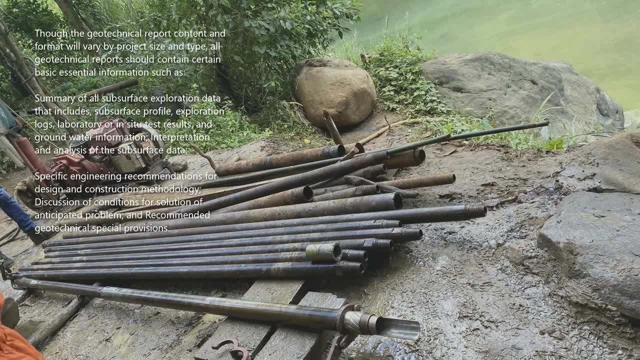 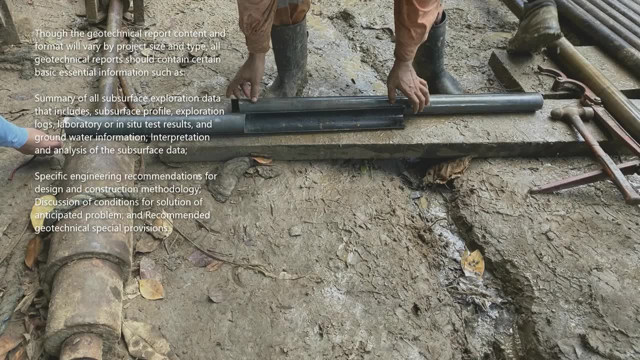 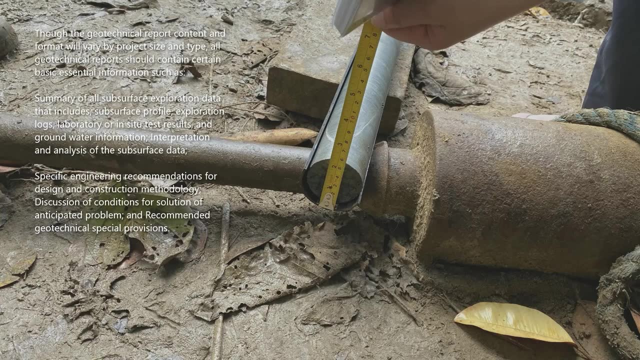 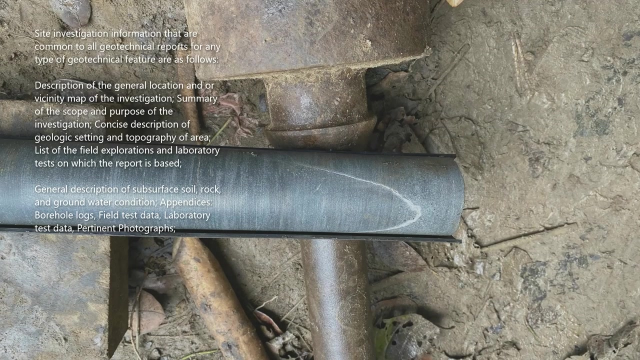 interpretation and analysis of the subsurface data, specific engineering recommendations for design and construction methodology. discussion of conditions for solution of anticipated problem and recommended geotechnical special provisions. Site investigation information that are common to all geotechnical reports for any type of geotechnical feature are as follows: 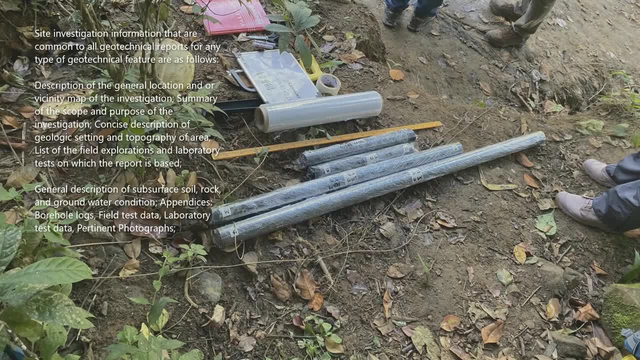 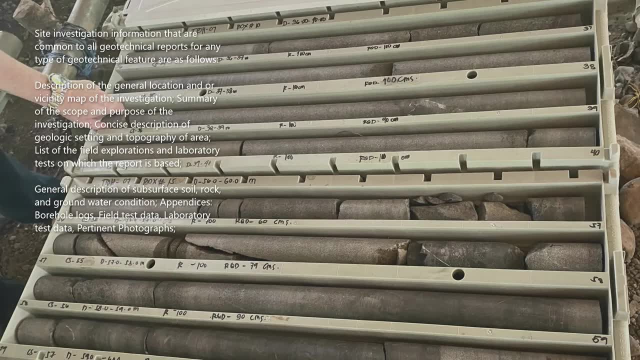 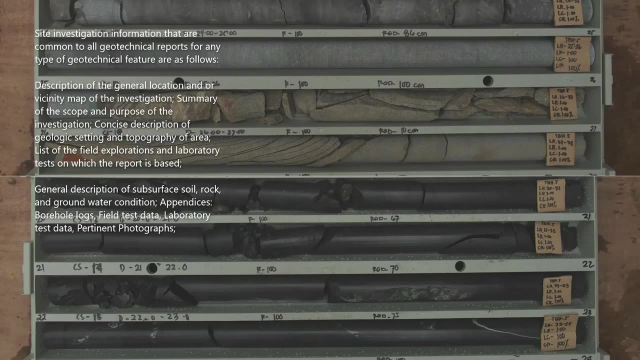 Description of the general location and or vicinity map of the investigation. Summary of the scope and purpose of the investigation. Concise description of geologic setting and topography of area. List of the field explorations and laboratory tests on which the report is based. General description of subsurface soil, rock and ground water condition. 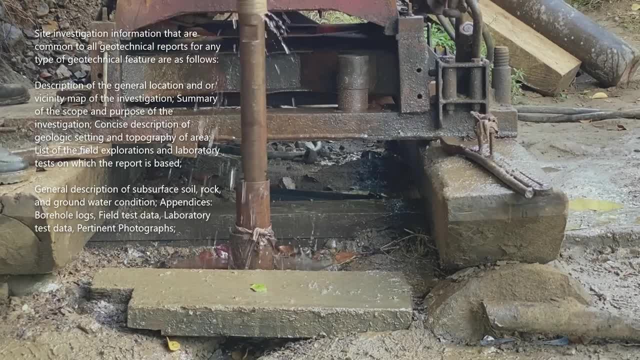 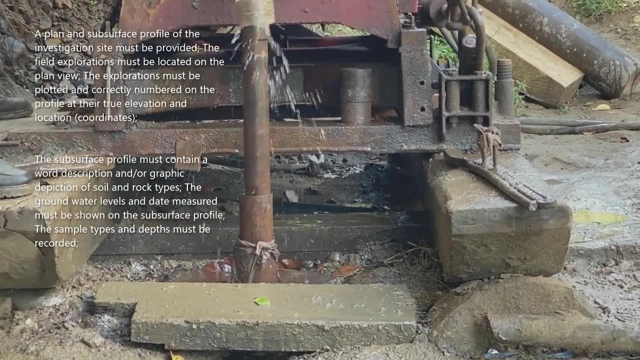 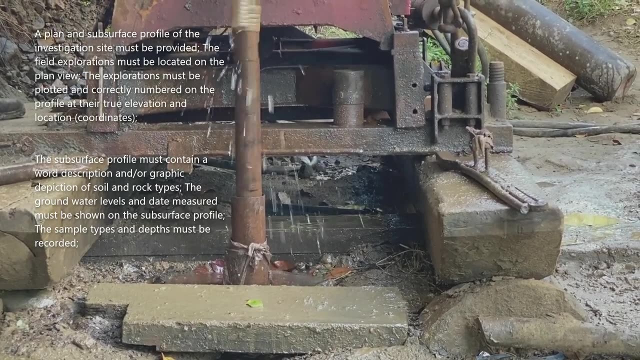 Appendices: borehole logs, field test data, laboratory test data, pertinent photographs. A plan and subsurface profile of the investigation site must be provided. The field explorations must be located on the plan view. The explorations must be plotted and correctly numbered on the profile at their true elevation and location. 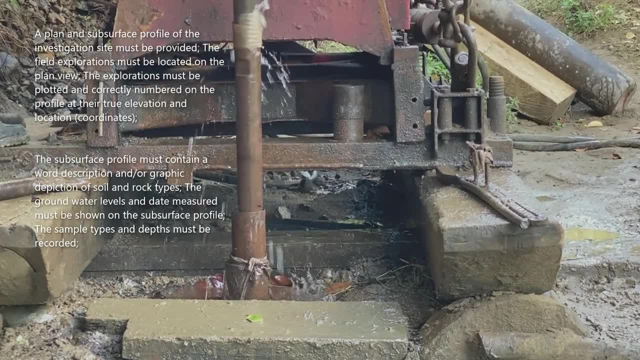 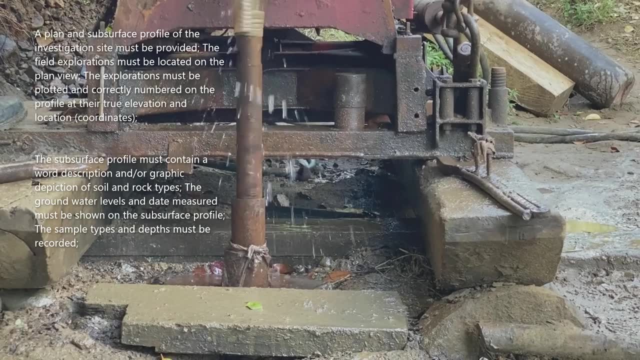 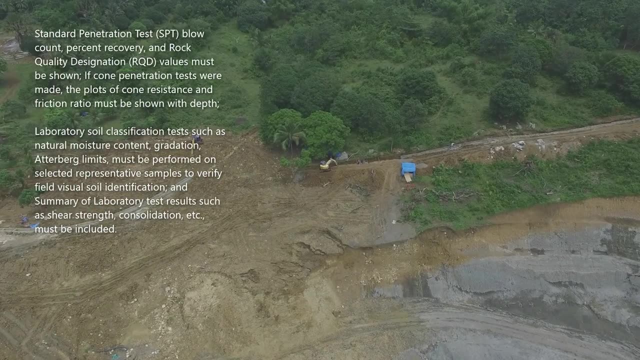 The subsurface profile must contain a word description and or graphic depiction of soil and rock types. The ground water levels and date measured must be shown on the subsurface profile. The sample types and depths must be recorded. SPT, blow count, percent recovery and RQD values must be shown. 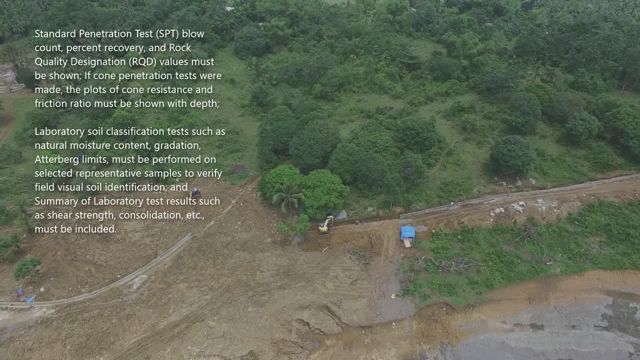 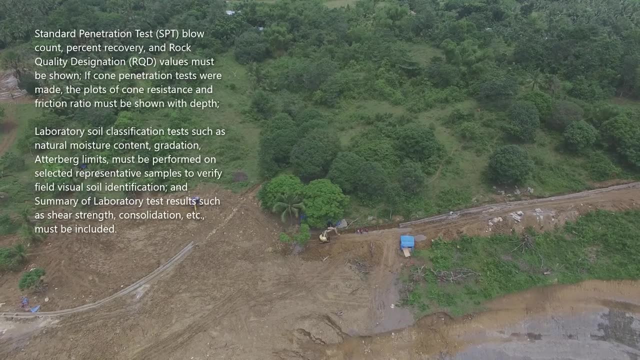 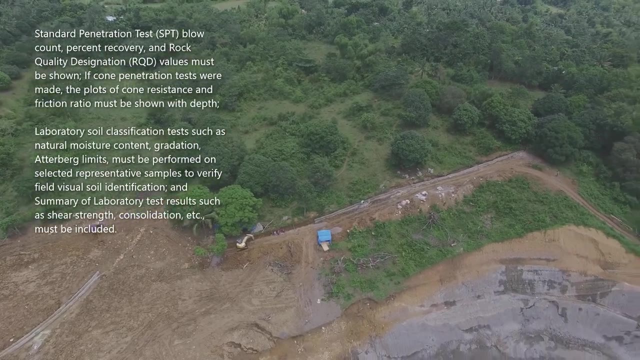 If cone penetration tests were made, the plots of cone resistance and friction ratio must be shown with depth Laboratory soil classification tests, such as natural moisture content gradation- Adderberg limits, must be performed on selected representative samples to verify field visual soil identification. 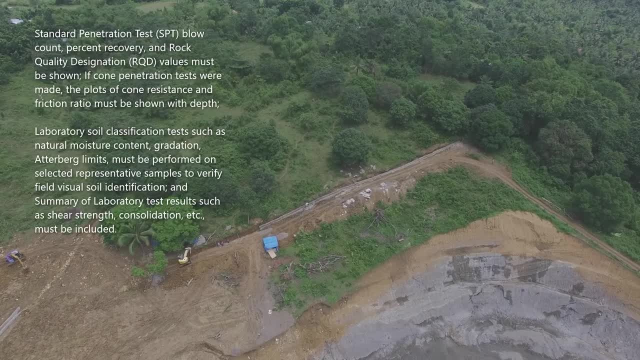 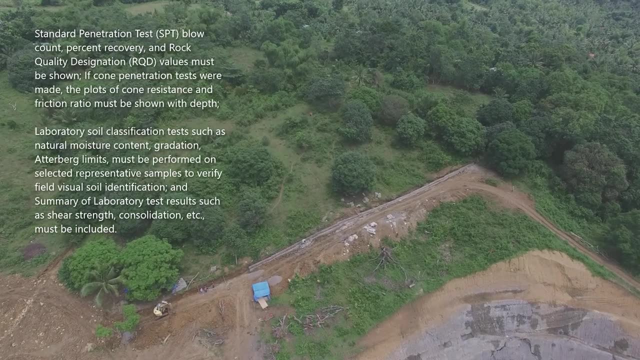 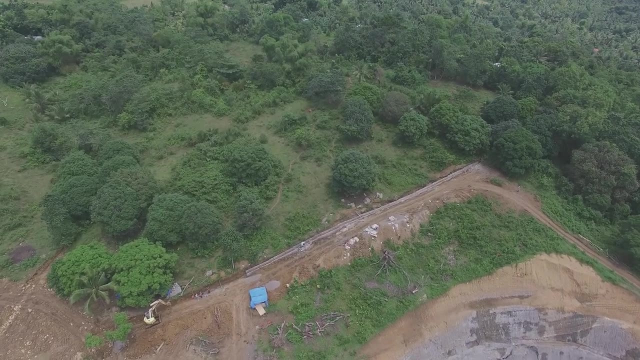 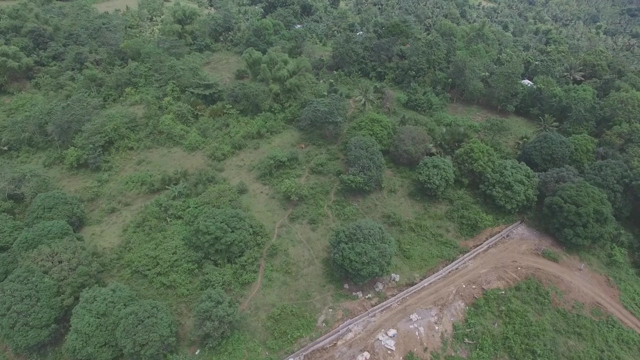 And summary of laboratory test results, such as shear strength, consolidation, etc. must be included. Thank you for watching. Please subscribe to our channel and press the bell icon to receive notifications of our latest videos. Thank you for watching. See you in the next video. Bye. 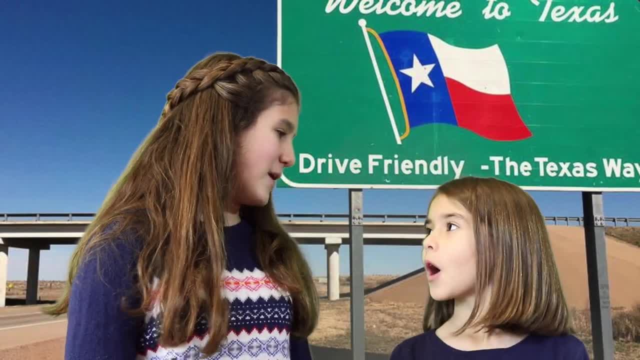 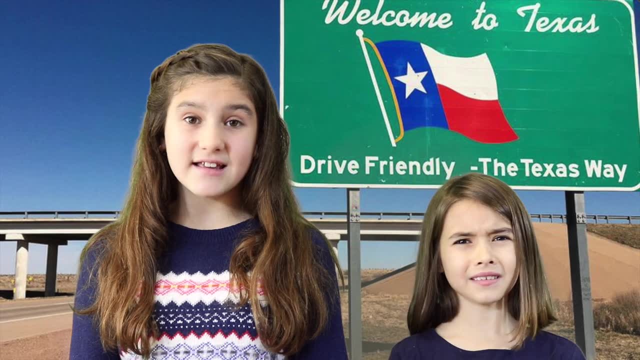 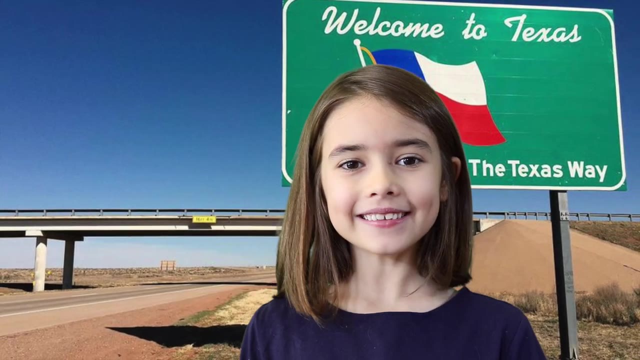 Hey everybody, Hey Quinn, guess what? What Cadence, You know how we're always talking about going places. Yeah, Let's go to Texas, Texas. Yeah, let's learn about Texas. Good idea: Texas is the second largest state in the USA. It is also the largest southern state. 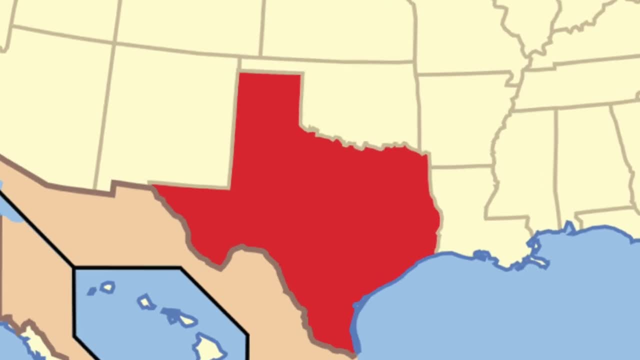 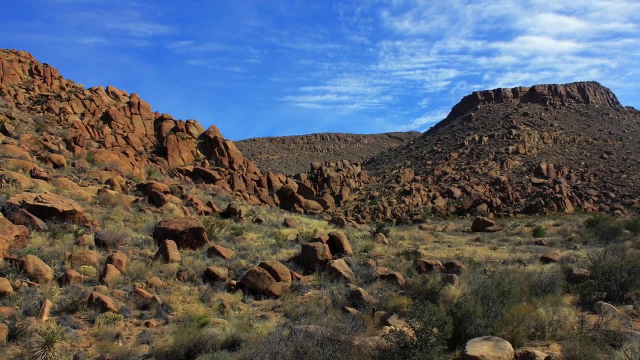 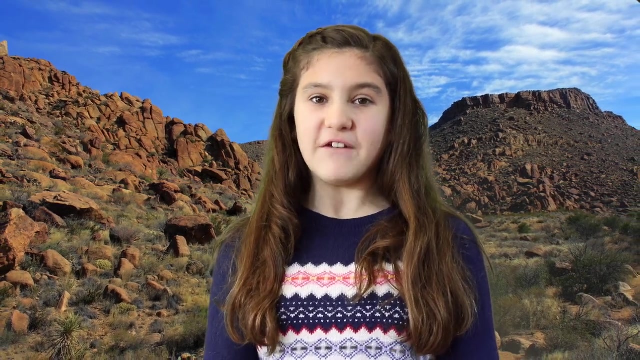 Its landscape includes deserts, systems of caves, mountains, canyons, forests and the Rio Grande River. The Rio Grande River is a river that forms the border between Texas and Mexico. Texas was first explored in 1528 by Spanish explorers on accident, when their ship sank off the coast. Texas did not become a colony until 1685.. France claimed it. Did you know? Spain then set up a rival colony in 1691? They set up a religious outpost in the eastern part of Texas. Spain did not return to Texas until 1716. 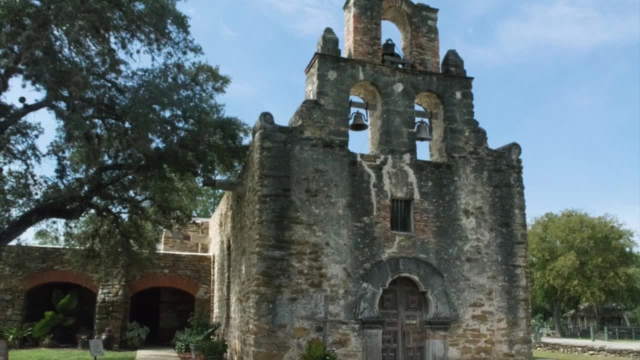 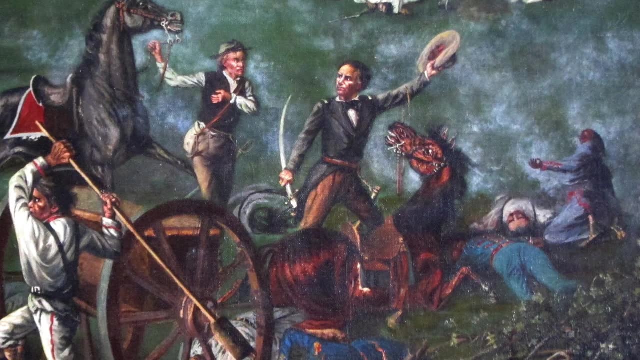 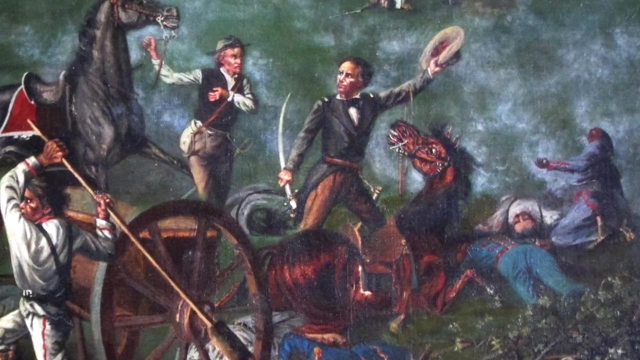 They came back to protect their colonies in the west from French forces. San Antonio was started two years later. The disagreement between the Spaniards and Native Americans in east Texas prevented many settlers from coming to Texas to make it their new home, To stop the violence as well as the numbers of Native American raids. 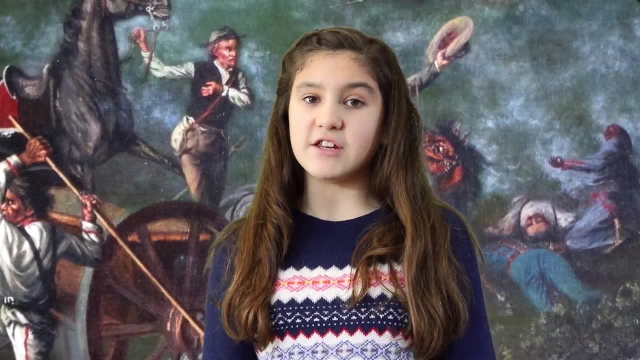 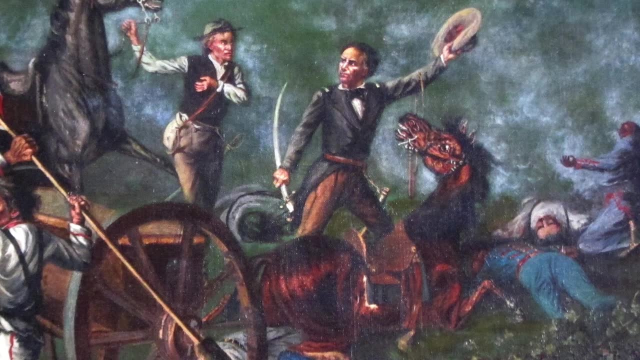 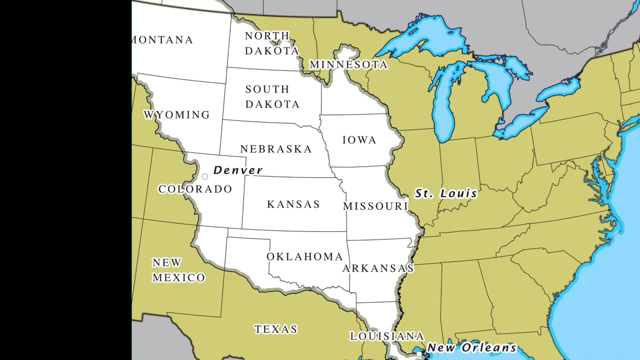 Spain called a truce between many tribes in 1745 and 1789.. But the tension got worse in Texas once the United States purchased a large piece of land from France in 1803.. This land was called the Louisiana Purchase. People began to wonder if Spain or the United States would actually claim Texas. 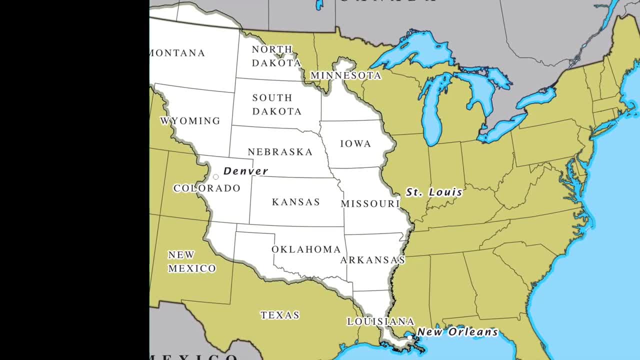 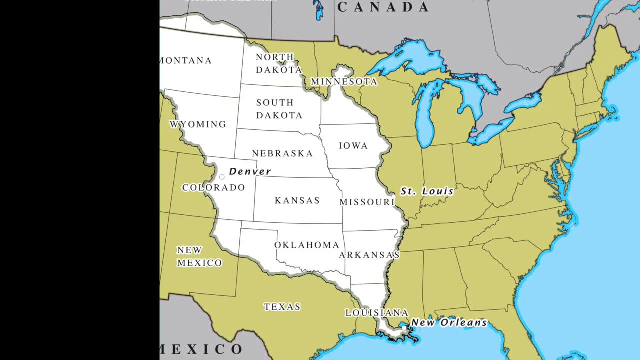 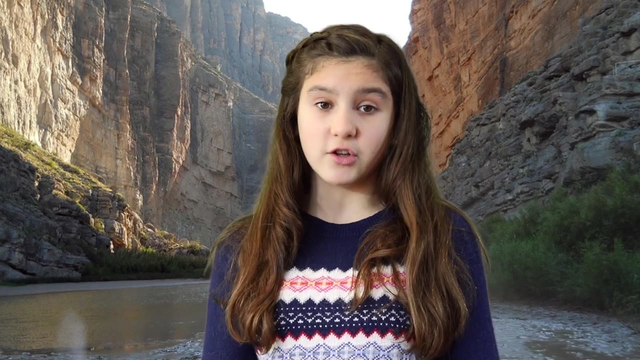 And when Mexico got its independence from Spain in 1821, Texas actually became a part of Mexico. They began calling the area Coahuila y Tejas. Americans and other settlers moved to Texas when Mexico allowed non-Spanish settlers to settle here.